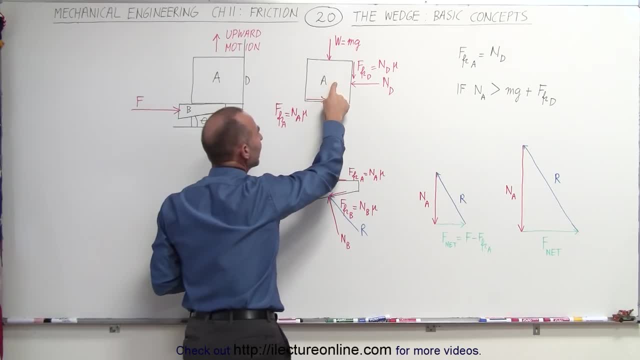 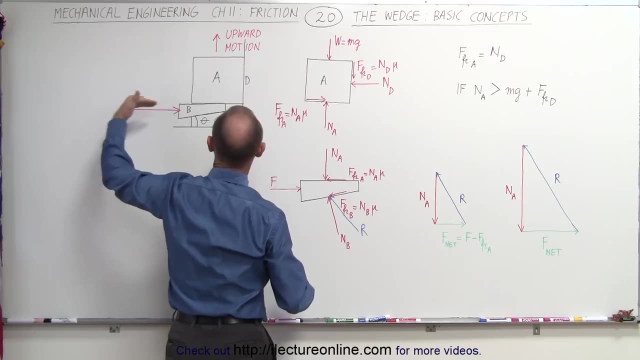 driving the wedge in here has to both lift up a and counterbalance the friction force at surface d. We can also see that the force driving the wedge in here will cause a friction force to exist between b and a which causes a force to act on a in the positive x direction. 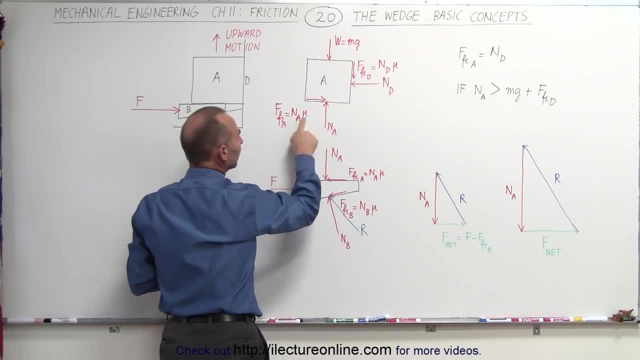 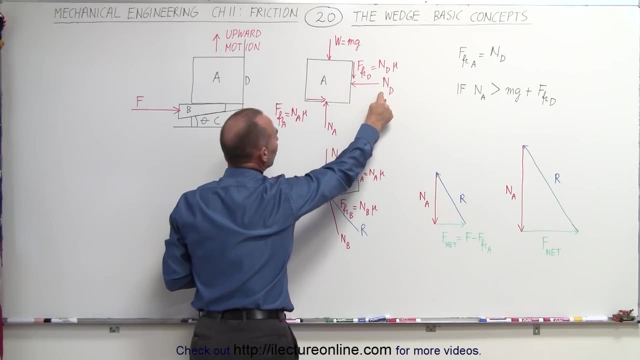 That's the friction force at a, which is the normal force at a times mu. That will then cause a normal force to exist on the back surface, here called the normal force at d, which then causes the friction force over there. The greater this friction force, the greater the normal force here. 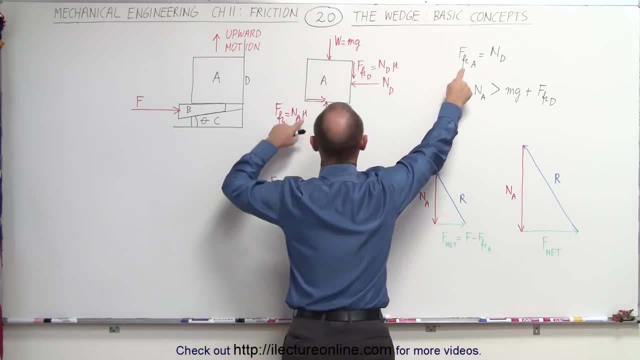 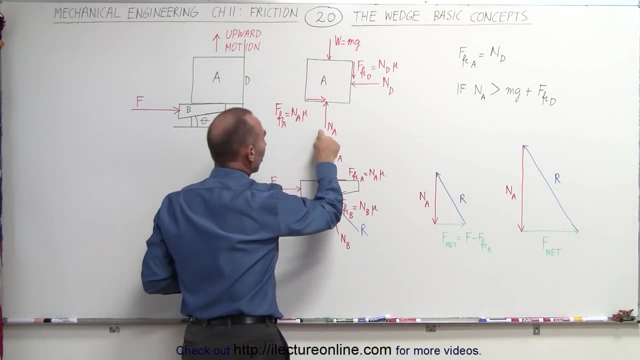 the greater the friction force there. Notice, the friction force at a is equal to the normal force at d And eventually, or finally, you can say that if n sub a is large enough to overcome both the weight of the wedge in here and the force on the other side of the wedge in here, You can also say: 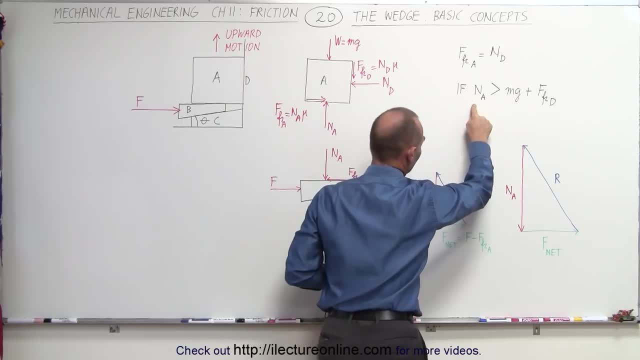 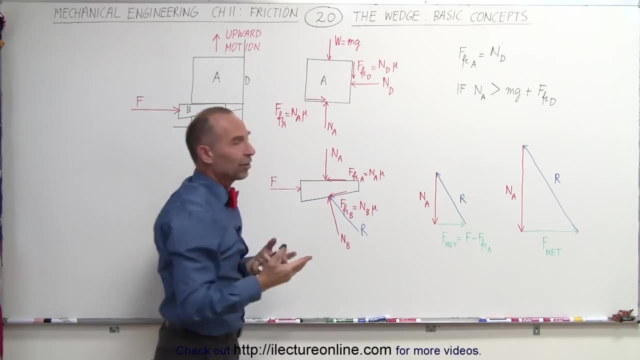 that the force of object a and the friction force at d. if n sub a is greater than the weight and the friction force, the object will go upward. So that's the ultimate objective here is to get a to go up to drive the wedge in there. If we look at the forces on the wedge here, notice we have n sub a also. 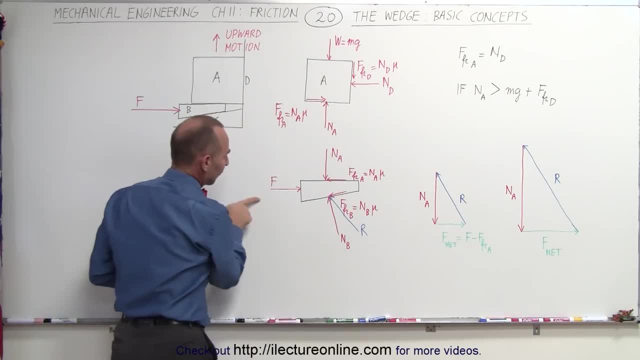 acting downward to the top surface of the wedge. We have the force trying to drive the wedge in and we have a normal force at the surface b. here, Notice, the normal force is slanted and we have an angle here relative to the horizontal. Typically those angles are fairly 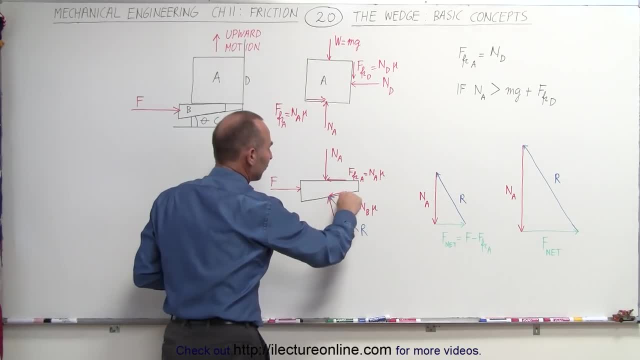 small Notice. there will also be a friction force at b against the wedge, and so there'll be a resultant force which is the vector sum of these two forces, the normal force at b and the friction force at b. Also notice: the magnitude of the friction force at a here is the same as the magnitude of the. 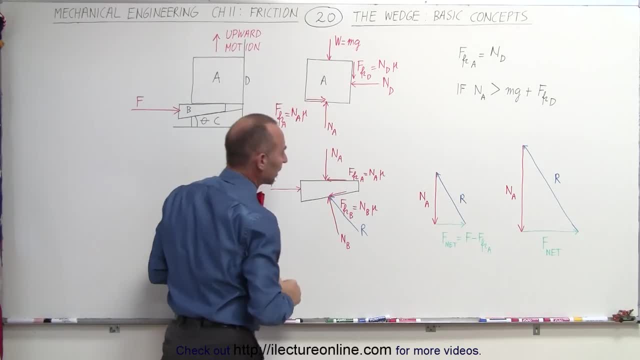 friction there, because these are forces sliding over one another Eventually. what we can now do is draw a diagram here of the force at a and the force at b. Notice that the force at a here is the forces acting on the wedge. We have the normal force acting downward, We have the resultant. 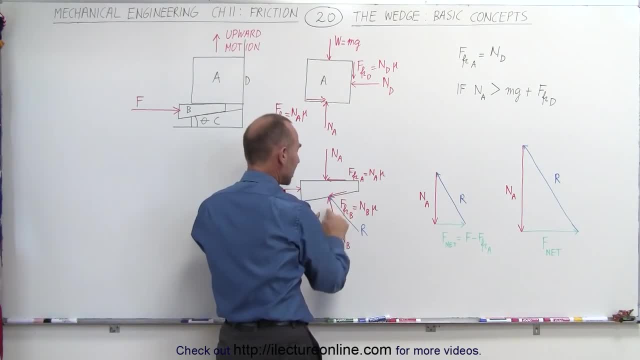 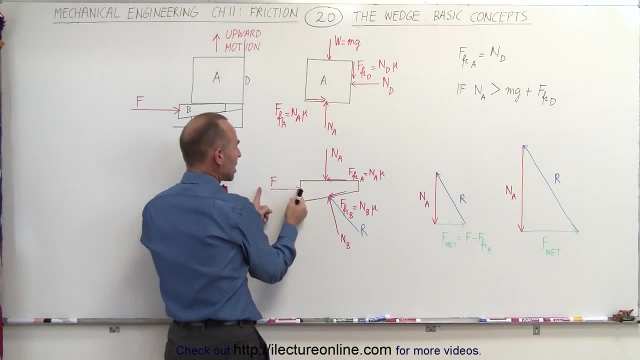 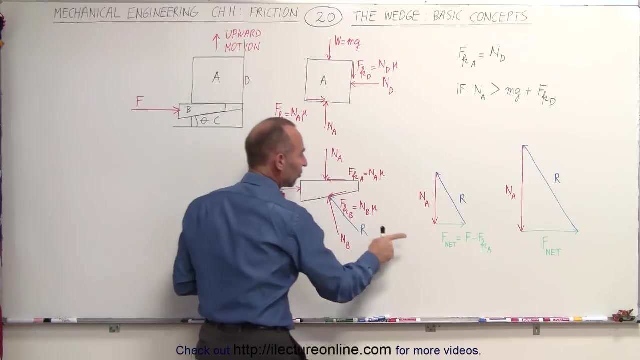 force at the bottom surface, which is the sum of these two forces right here, and then we have the net force driving the wedge in. The net force will be equal to the force here that's pushing against the wedge, minus the friction force there which is pushing back. So the net result of that is the net.